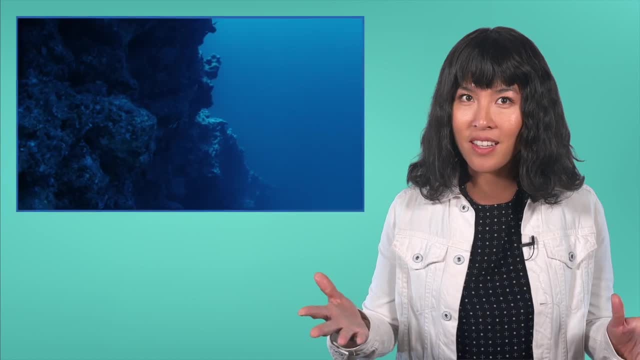 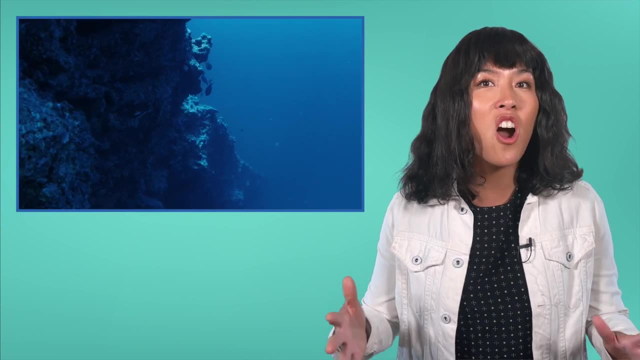 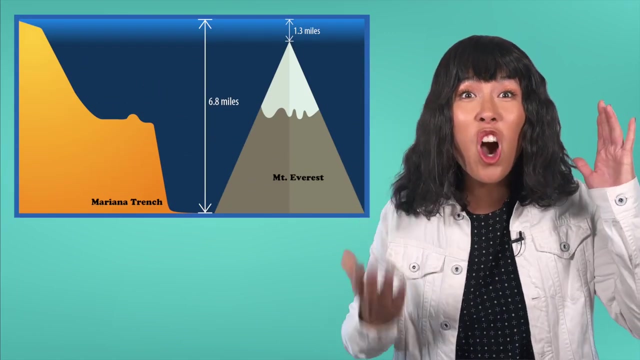 the sea like the Mariana Trench. At nearly 7 miles below the ocean's surface, the pitch black, ice-cold waters of the Mariana Trench are the deepest place on Earth. In fact, it's so deep that if you submerged the world's tallest mountain into the Mariana Trench, 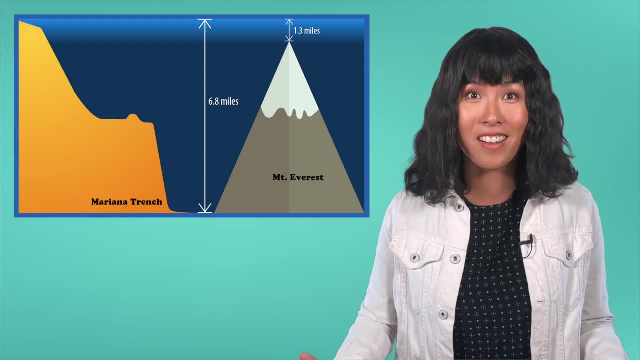 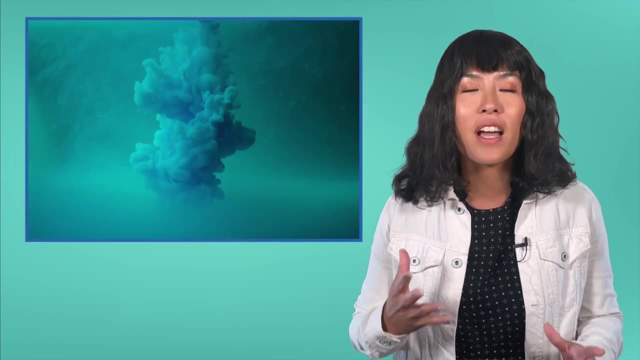 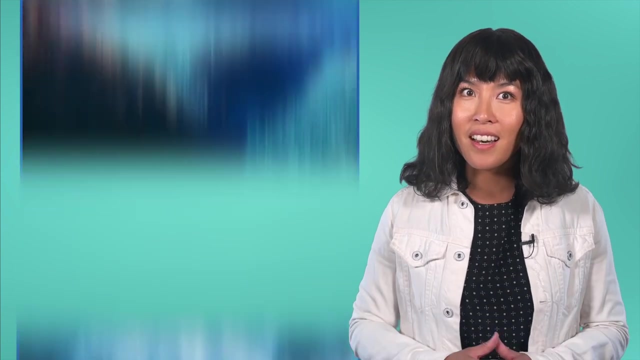 it would still be nearly a mile and a half underwater. And the ocean floor isn't only home to deep sea trenches either. You can also find volcanic activity, mountain ranges and brand new pieces of the Earth's crust. So what's going on under the sea that creates all these different geological features? And 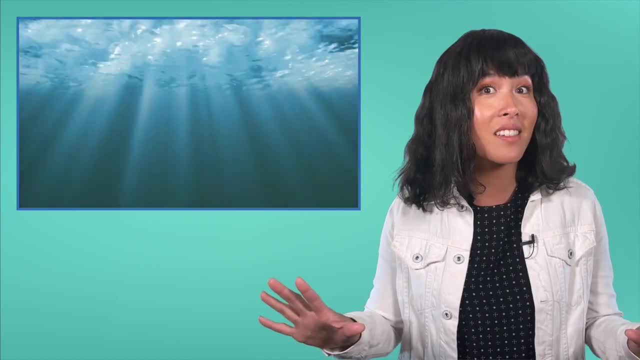 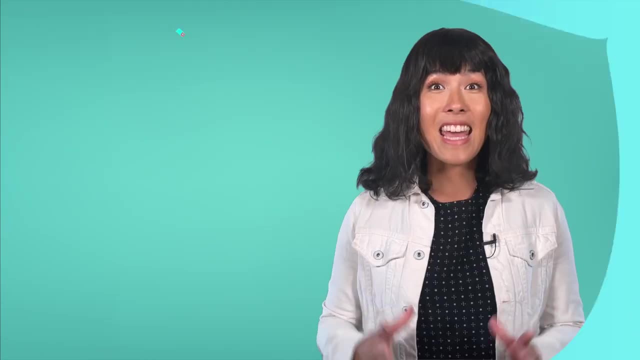 how is it different from the processes that shape the land? Today, we'll be diving into the depths of plate tectonics to answer these questions and more. In this lesson, we're going to Explain how plate tectonics create mid-ocean. 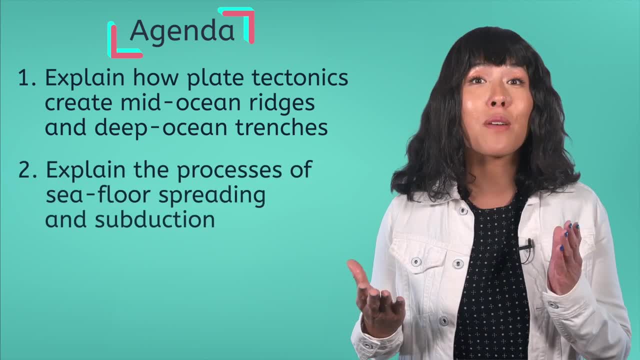 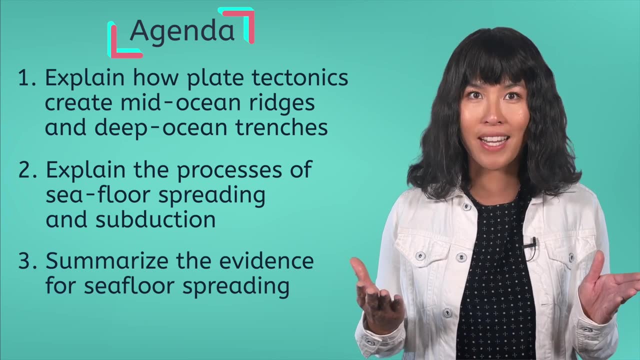 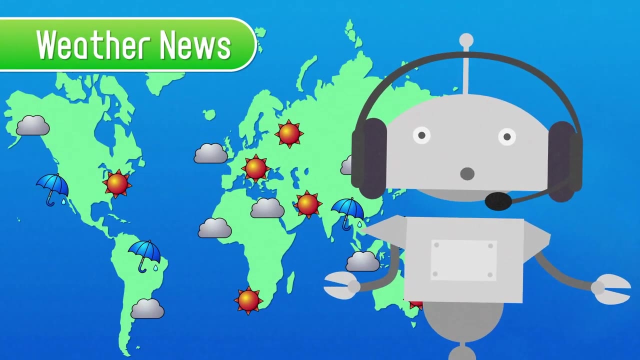 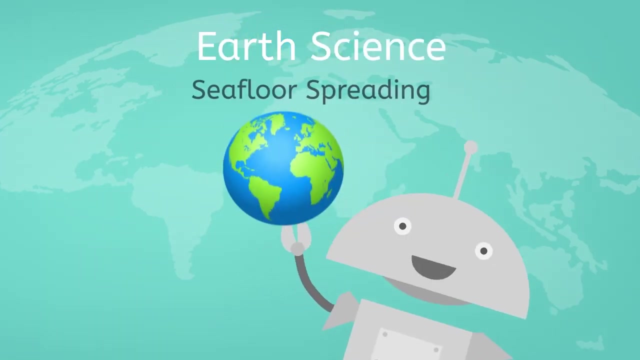 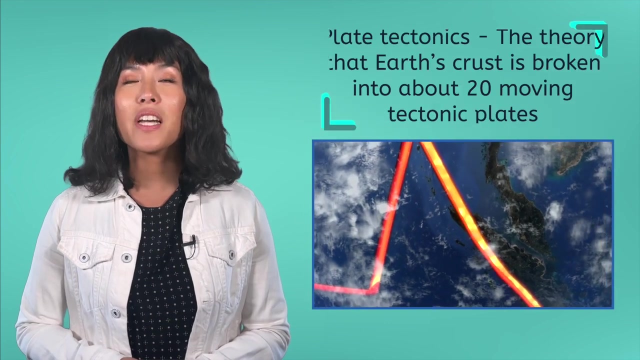 ridges and deep-ocean trenches, Explain the processes of seafloor spreading and subduction, And summarize the evidence for seafloor spreading. Let's get started. Before we jump in, let's review a bit about plate tectonics. The theory of plate tectonics states that the Earth's crust is broken up into about. 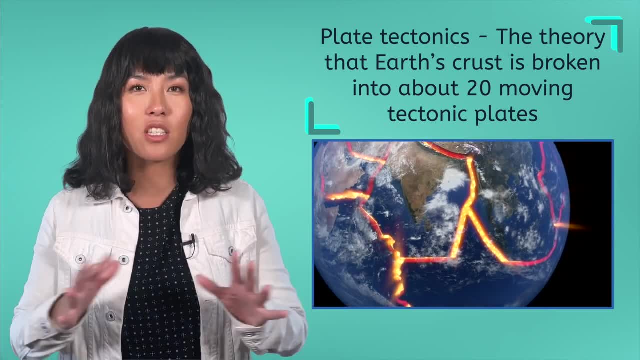 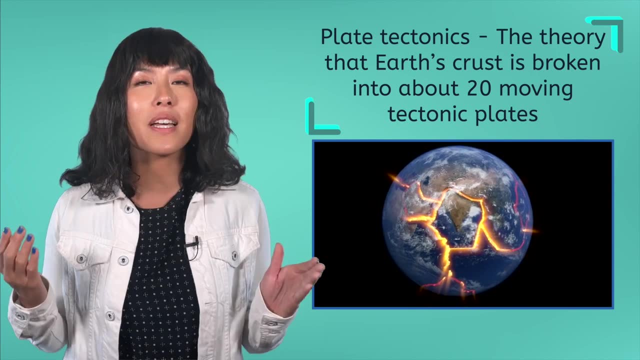 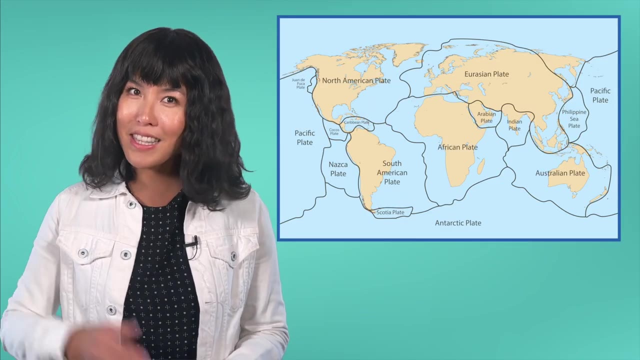 20 segments, called tectonic plates, that slowly drift around the planet's surface, moving the continents with them. However, not all of the plates that cover Earth's surface are the same. There are two kinds of tectonic plates. Take a look at this map. What do you think? the? two kinds of plates could be. Pause the video here and write your answer in the comments. If you're interested in learning more about plate tectonics, please subscribe to our YouTube channel and click the bell icon to be notified when we post a new video every week. Take a look at this map. What do you think the two kinds of plates could be? Pause the video here and write your answer in the comments. Take a look at this map. What do you think the two kinds of plates could be? Pause the video here and write your answer in the comments. Take a look at this map. What do you think the two kinds of plates could be? Pause the video here and write your answer in the comments. Take a look at this map. What do you think the two kinds of plates could be? Pause the video here and write your answer in the comments. Take a look at this map. What do you think the two kinds of plates could be? Pause the video here and write your answer in the comments. Take a look at this map. What do you think the two kinds of plates could be? Pause the video here and write your answer in the comments. 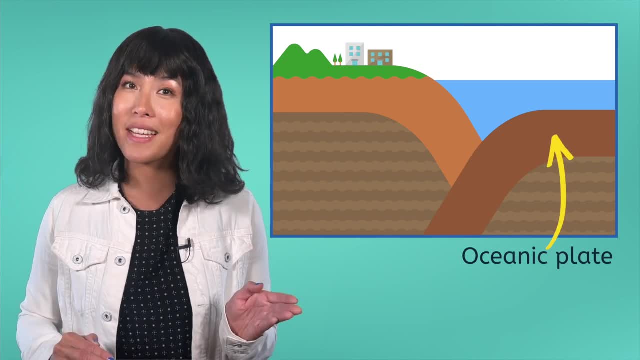 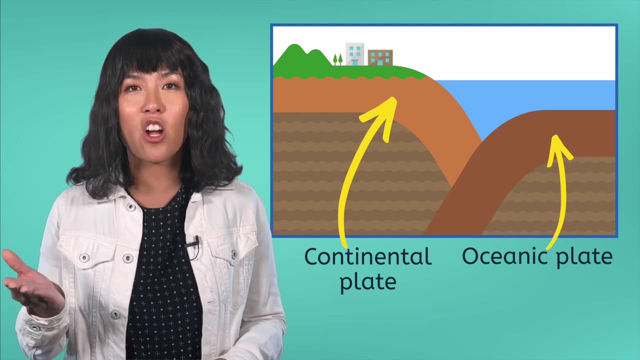 Take a look at this map. What do you think the two kinds of plates could be? Pause the video here and write your answer in the comments. ocean are called oceanic plates, while plates beneath land masses are called continental plates. continental plates are much, much thicker than oceanic plates, but oceanic plates are made out. of denser, heavier rocks. when a continental plate and an oceanic plate crash into each other at a convergent boundary, the denser oceanic plate slips underneath the continental plate. this makes the seafloor buckle and change shape, often forming deep oceanic trenches, as it's pulled down, like the. 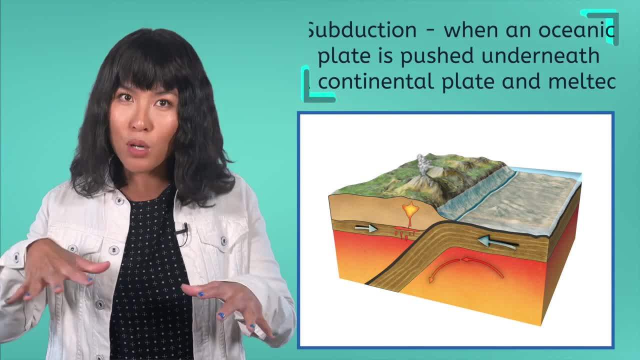 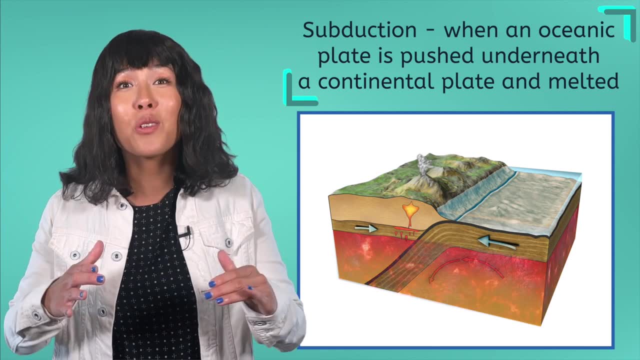 mariana trench. when an oceanic plate is pushed down underneath a continental plate, it's called subduction. during this process, the plate melts back into the earth's mantle. because of subduction. the tectonic plate is pushed back into the earth's mantle. because of subduction, the tectonic plate. 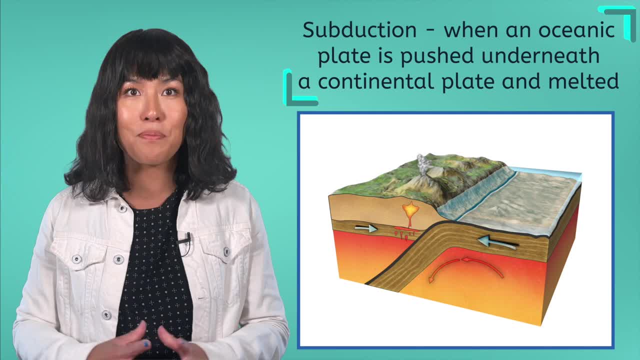 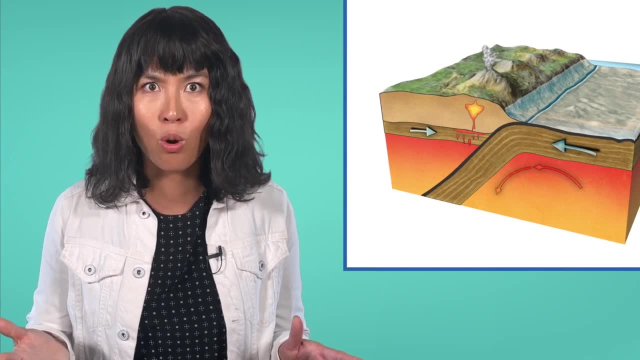 is pushed back into the earth's mantle. because of subduction, the tectonic plates that carry earth's oceans are constantly being destroyed, so you might be wondering what's going to happen to the seafloor if it's slowly being absorbed back into the planet. if you dive deep enough, can you reach. 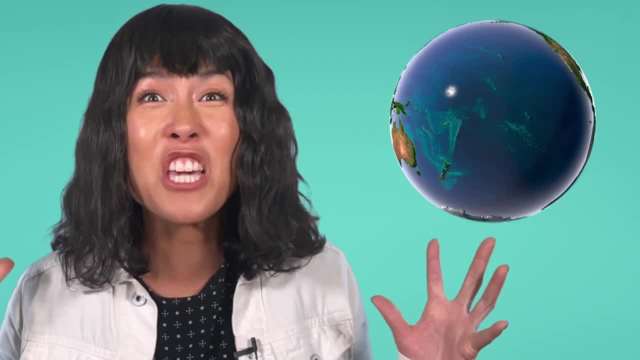 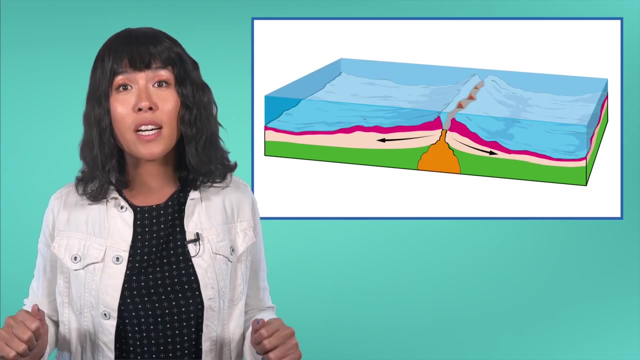 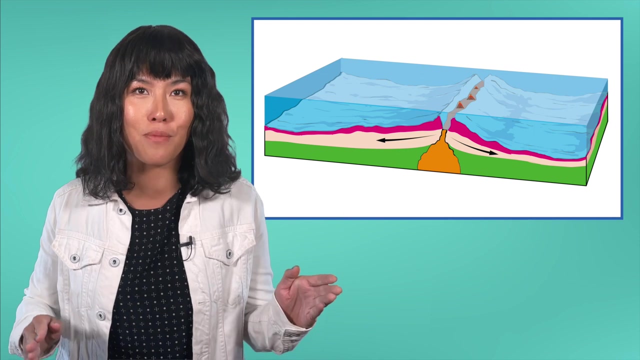 the mantle? what will happen to the ocean when all of the oceanic plates slip beneath the continental plate? to answer these questions, well, we need to leave the subduction zone at this convergent boundary and head to a divergent boundary between two oceanic plates instead. 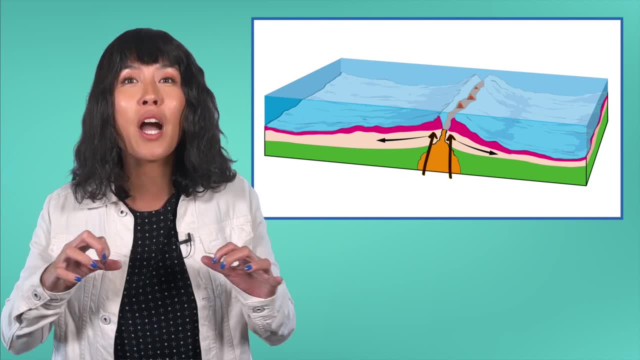 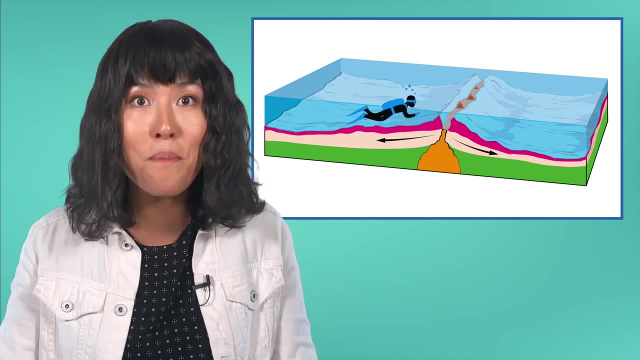 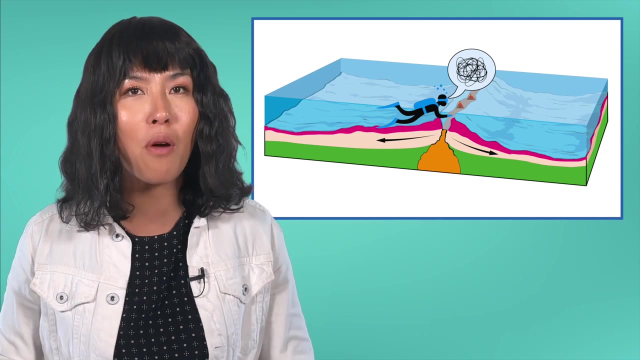 these boundaries are places where the ocean floor is pulling apart, but even as the plates separate, it doesn't just create a gap in the crust where you could swim down to the mantle. that's because these divergent boundaries between oceanic plates are the site of a process called seafloor spreading. 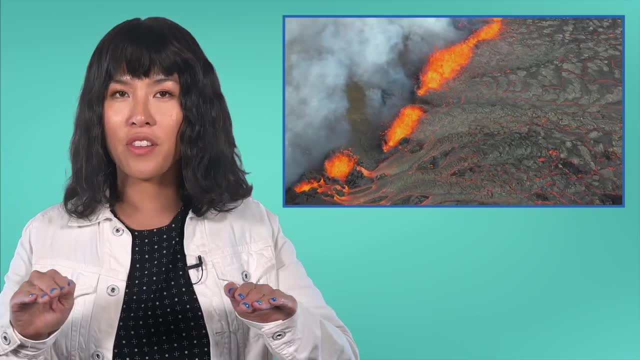 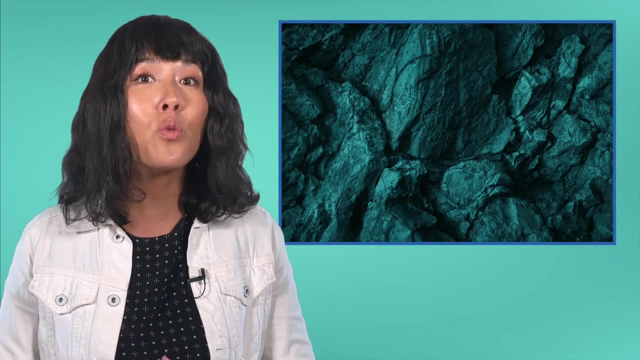 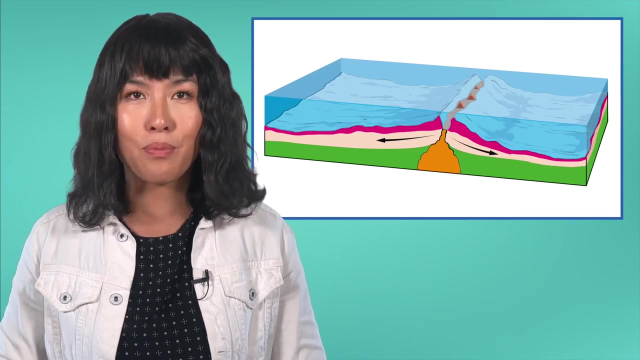 as the two oceanic plates pull apart from each other, magma from the planet's mantle rises up to fill the empty space. when this magma cools and hardens into igneous rock, it bridges the gap between the plates. this creates new oceanic plates to replace the ones being melted down. 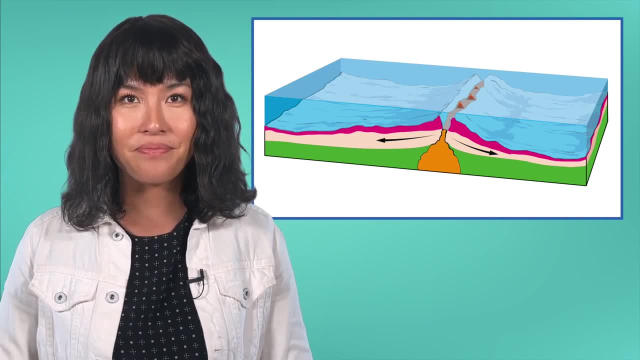 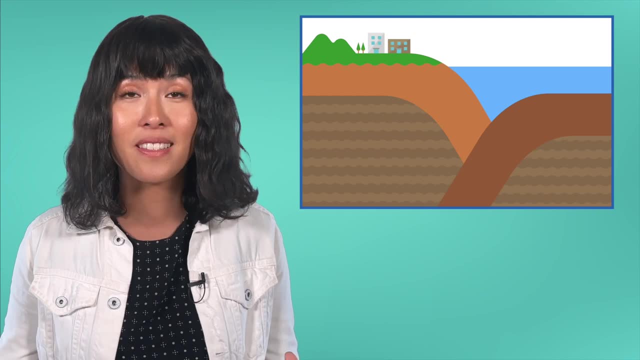 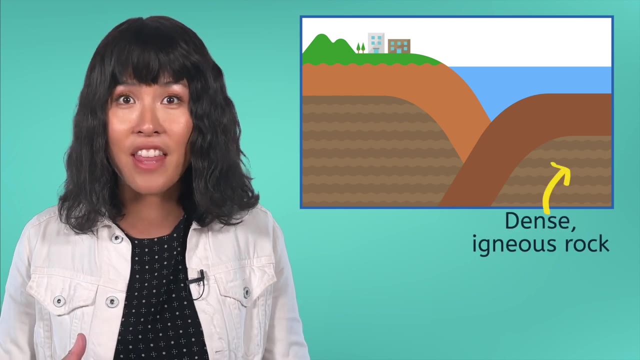 during subduction at convergent boundaries. at the same time, the process of seafloor spreading is why subduction happens in the first place. oceanic plates are denser than continental plates because they're made of igneous rock, and they're made of igneous rock because of the magma that 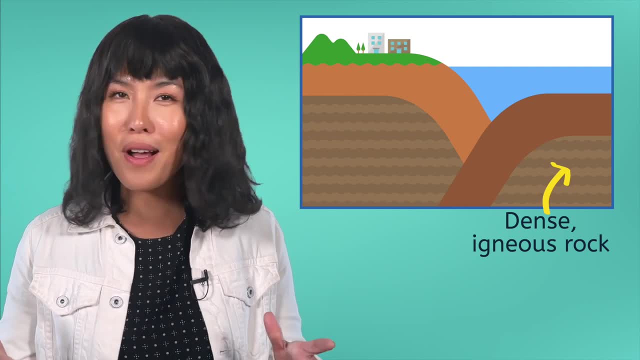 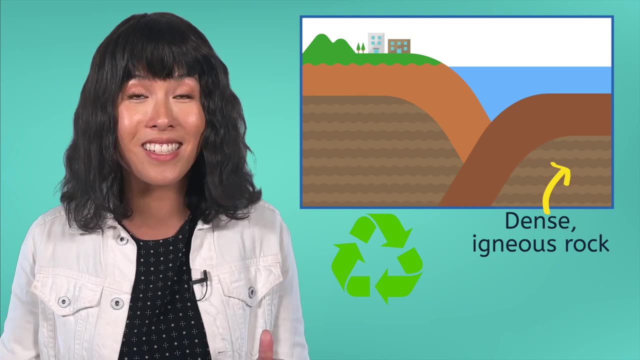 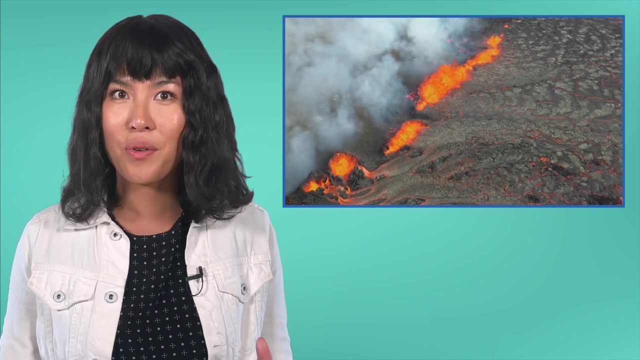 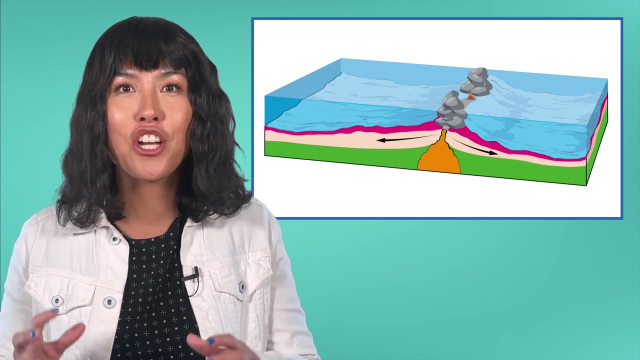 wells up during seafloor spreading. see how the processes that shape the earth are all interconnected. even the earth recycles its own crust as this magma cools and hardens. it does more than just create new oceanic plates, though. new rocks tend to really pile up along the edges of the plates, creating entire undersea. 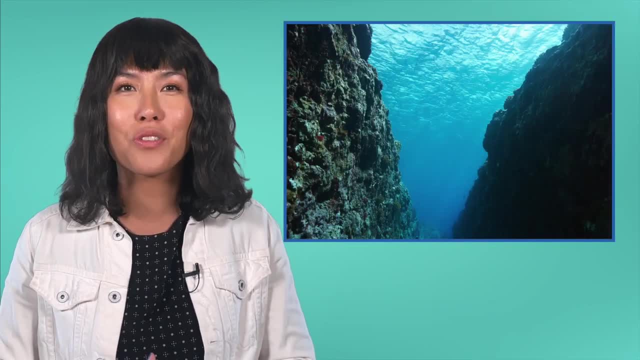 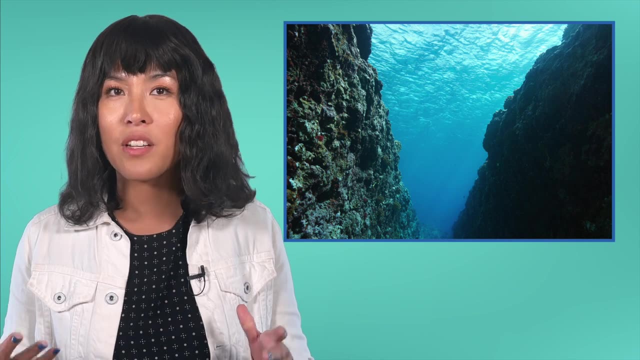 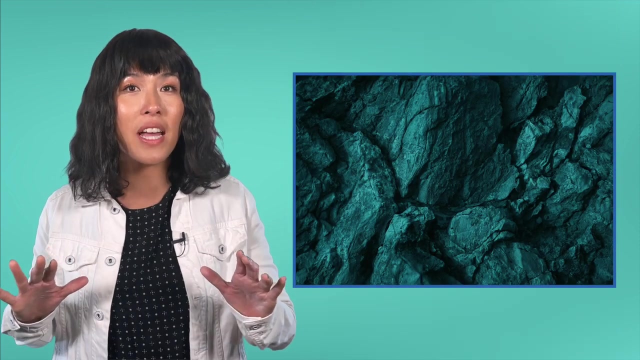 mountain ranges, known as mid-ocean ridges now, sea floor spreading might seem like a wild idea, but geologists have found lots of evidence that supports it. firstly, these mid-ocean ridges are made of basalt, an igneous rock. this basalt also tends to be 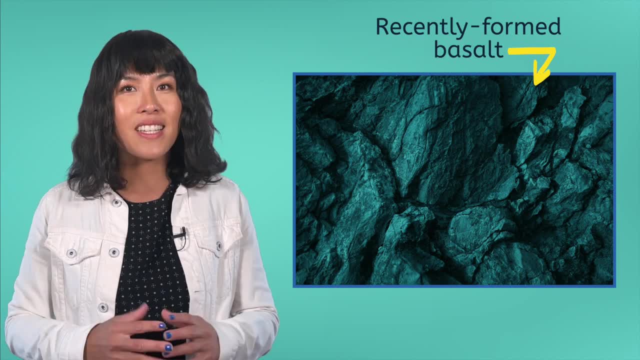 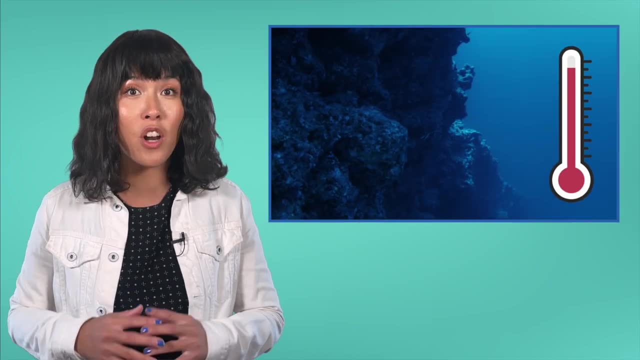 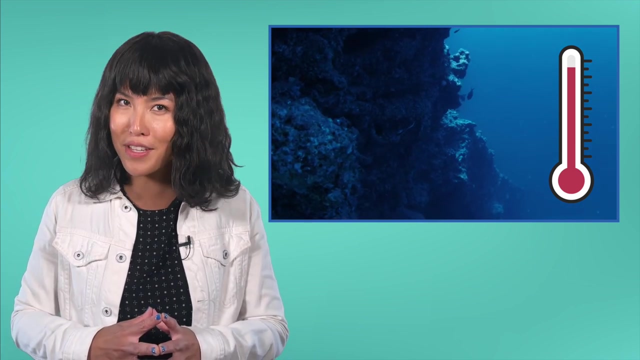 much younger than the ocean floor around it, telling us that it formed recently in geological terms. they've also discovered that the temperature of the water around mid-ocean ridges tends to be warmer. what do you think makes this a convincing piece of evidence? pause the video here and write. 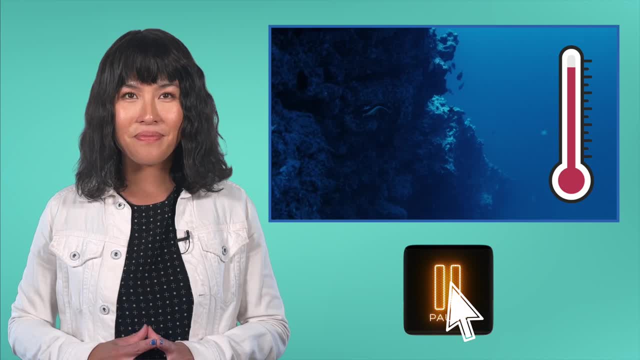 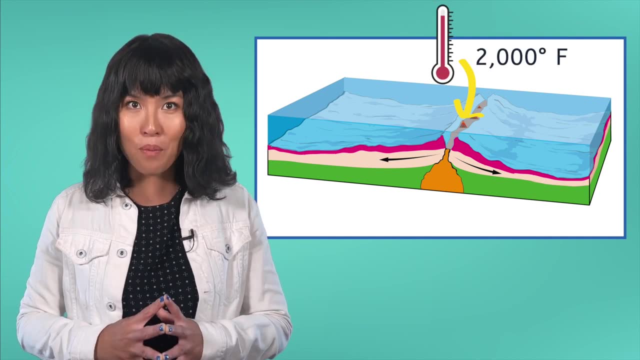 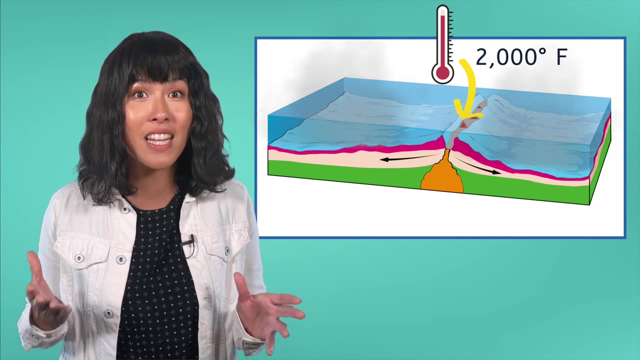 your answer in your guided notes, remember. even the upper parts of the mantle are nearly 2 000 degrees higher than the lower parts of the mantle. so the magma that wells up from the planet's interior during seafloor spreading is hot enough to raise the temperature of the ocean nearby. 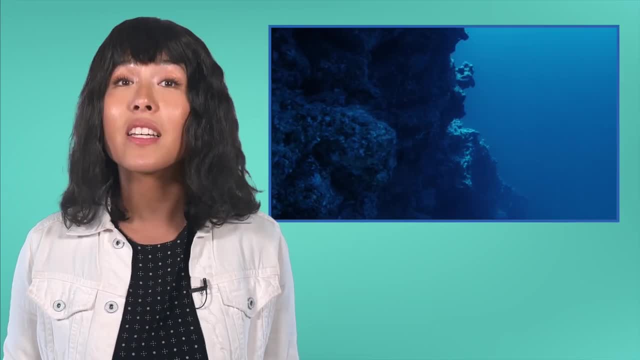 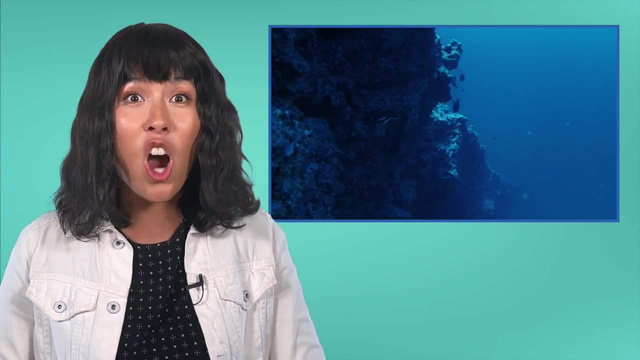 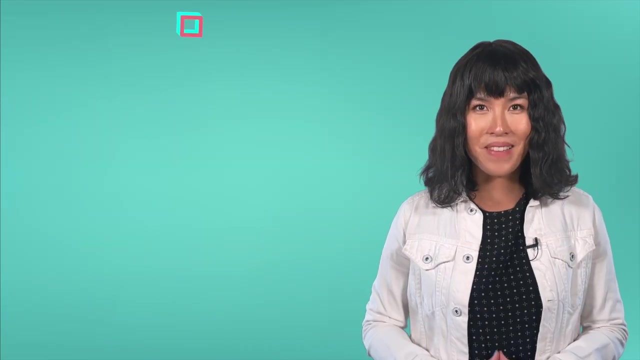 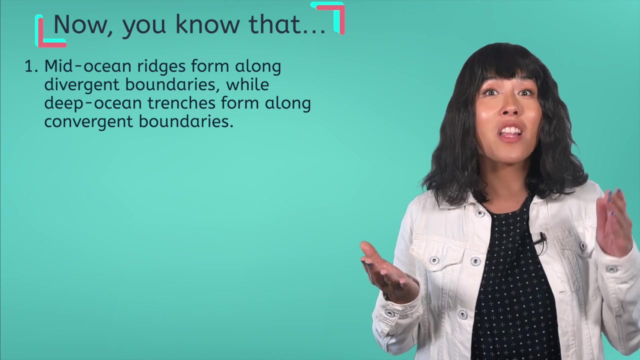 geologists agree that the evidence for seafloor spreading is pretty convincing. it helps us understand yet another way that interconnected geological processes are constantly shaping our planet. so let's go over what we learned today. now you know that mid-ocean ridges form along divergent boundaries, while deep ocean trenches form along convergent boundaries. 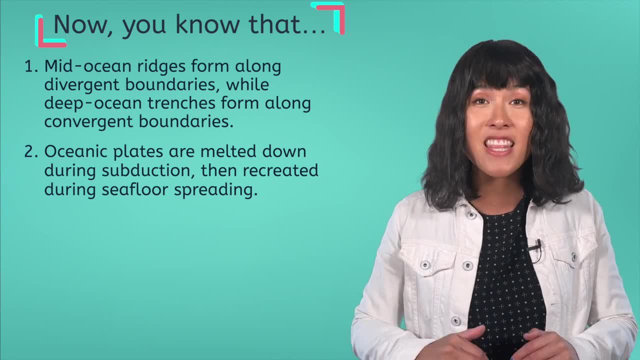 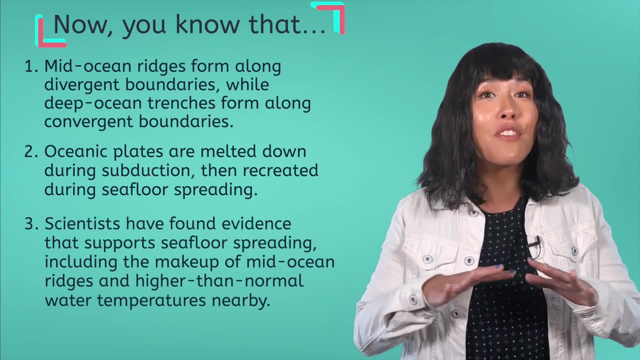 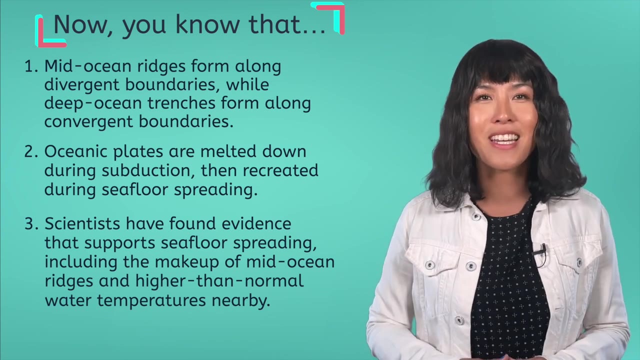 oceanic plates are melted down during subduction, then recreated during seafloor spreading, and scientists have found evidence that supports seafloor spreading, including the makeup of mid-ocean ridges and higher than normal water temperatures nearby. be sure to check out the engaging games and thought-provoking experiences of the mid-ocean ridges and the seafloor ridges.